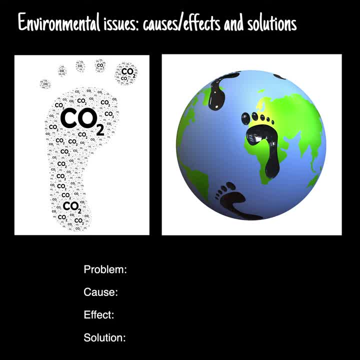 Number 1.. The first environmental problem that we want to talk about is our carbon footprint. What is our carbon footprint, Jenny? This is our CO2 emissions. It's caused by the use of fossil fuels for transportation. People are driving cars and flying in planes wherever. 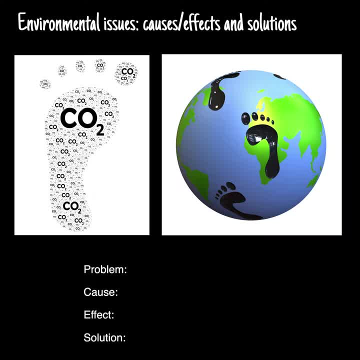 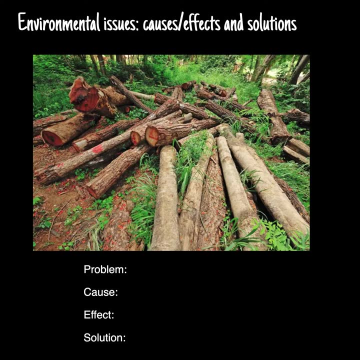 they want to go. And the effects, Aria? The effect is climate change and extreme weather. What are some solutions? Ashley, The solution is for people to use public transportation and travel less- Number 2.. Okay, let's move on to the 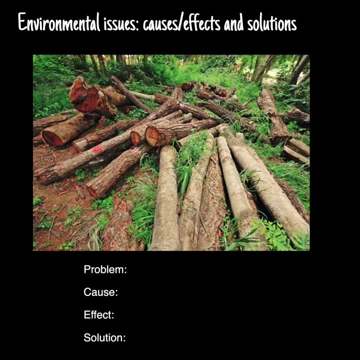 problem of deforestation Causes. anyone, Rosa, go ahead? This is caused by the cutting down of trees. Thank you, Rosa. William, the effects? The effects include floods, loss of wildlife, lower soil quality and so on. Emily, how about the solution? The solution is to grow trees and 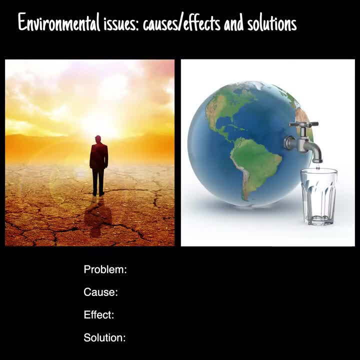 protect forests- Number 3.. The problem is the water crisis. There is a shortage of clean water, Okay, Monica. This is caused by overuse of water by factories and farms. The rivers are polluted And global warming Means some parts of the world are becoming drier. Prabhat, do you want to talk about effects? 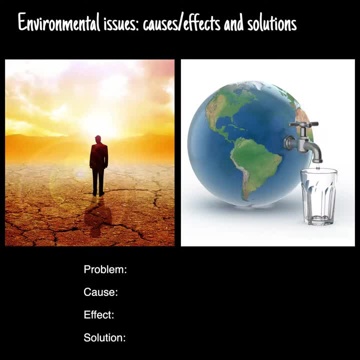 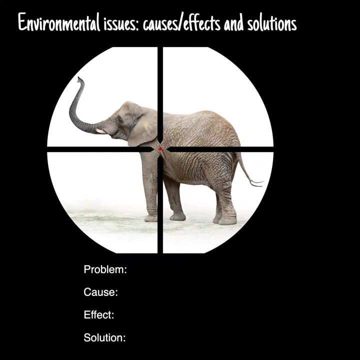 Yes, The effects include health problems and water shortages for farming and industry and actually for everyone. Clara, what is the solution? The solution is to manage water resources and protect forests- Number 4.. The next problem is hunting- Cora turn. This is caused by people who go hunting for sport And some animal products such as ivory. 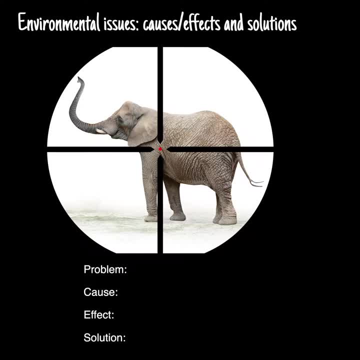 can be sold in many countries. That's right, And the effect is the loss of endangered wildlife such as elephants and tigers Amber. what about solutions? I think the solution is laws against hunting and effective enforcement of laws Number 5. Okay, 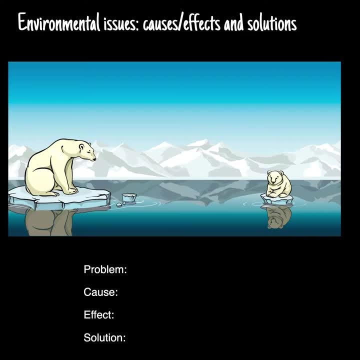 On to the problem of the melting ice cap. Everyone knows this is caused by global warming Right, And the effect is the rising level of the ocean, the loss of polar ice caps and the loss of wildlife such as polar bears. Yes, And I believe the solution is: all countries should try to reduce. 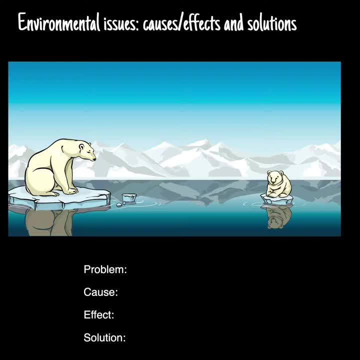 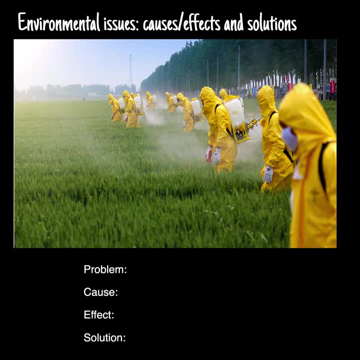 carbon emissions. Thank you, Eric, Number 6.. The problem is using toxic sprays for agriculture and farming, Brandon. This is caused by farmers trying to protect plants against pests and disease. All right, Elizabeth, tell me about the effects. One effect is the accidental killing of wildlife. 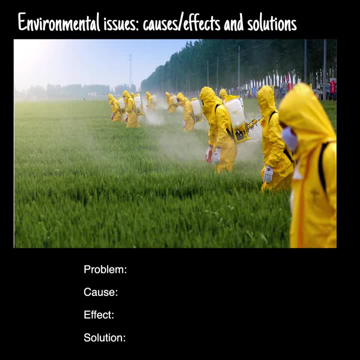 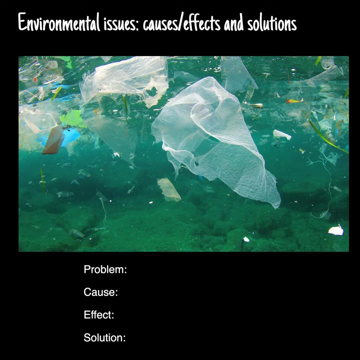 Also, toxic sprays and insecticides are dangerous for workers. Not only that, the farms may sell contaminated produce. Eric, do you have another solution? The solution is simple: Ban chemical and toxic sprays. Number 7. Everyone is familiar with this problem. This problem is plastic waste. Oh good, Liam. 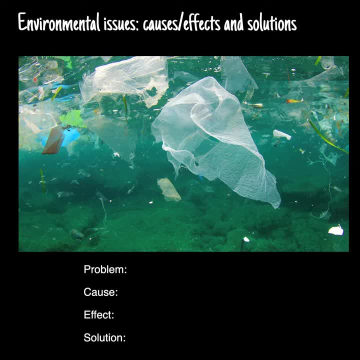 This is caused by the convenience of using plastic bags in shops and supermarkets. Mitchell, what are the effects of too many plastic bags? The effect is the killing of sea life and polluting of the oceans. Leah, give me a solution. The solution is persuade supermarkets and shops to stop using plastic. 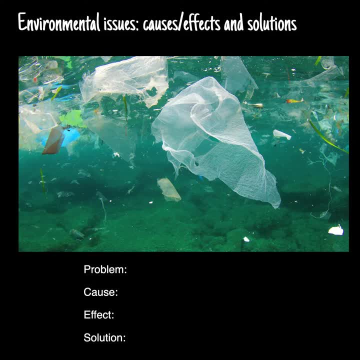 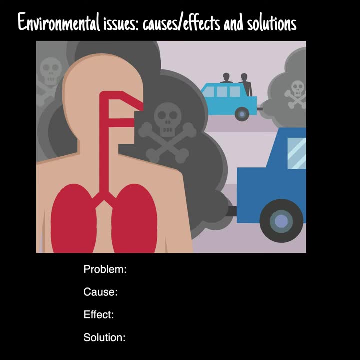 or legislate to stop them? Number 8.. The last problem is air pollution in our cities. Brandon, do you live in the city? Yes, I live downtown and sometimes I can't breathe. Air pollution is caused by people using cars, buses and trucks that rely on fossil fuels- Cora, how do you feel about this problem? 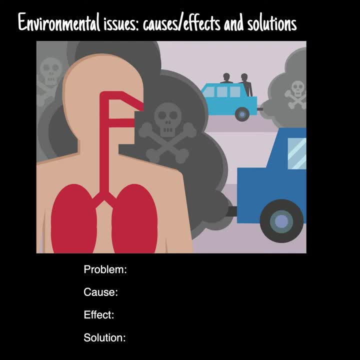 Well, air pollution has a bad effect on our health. Many people in cities have respiratory problems And, of course, it contributes to global warming. Okay, Elizabeth, what do you suggest as a solution? The solution is emissions controls for cars. We need alternative kinds of transportation.